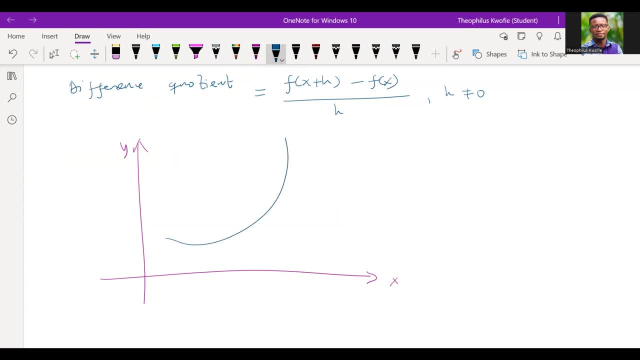 Let's call this X, Let me call this Y, If this is my. I have a curve. I have a curve as this. So the problems we are confronted with in life is as if it's like a curve as this. Okay, 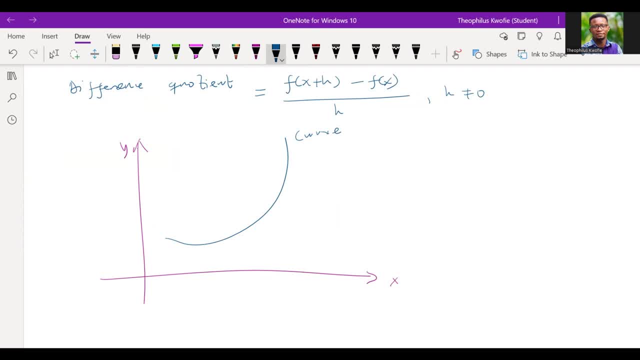 So this is our curve that we are talking about, of which, I said, is nonlinear. Okay, So this is a problem we want to solve, But then this is a mindset. I want us to have this mindset that, for us to solve this curve, we want to make sure. 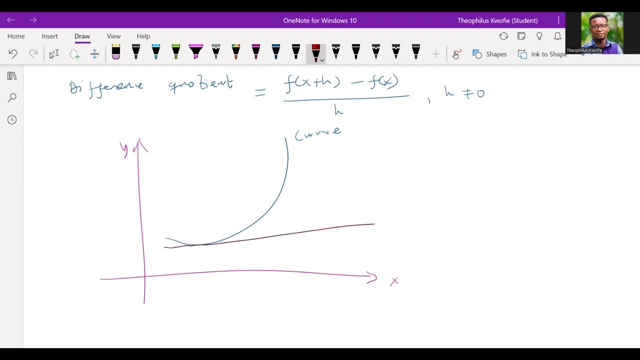 that the problem becomes as smooth as this, In other words, becomes aligned as this. So let me call this as my T. Okay, So this is a curve and this is a line. Now suppose this is a point. Let's call it. 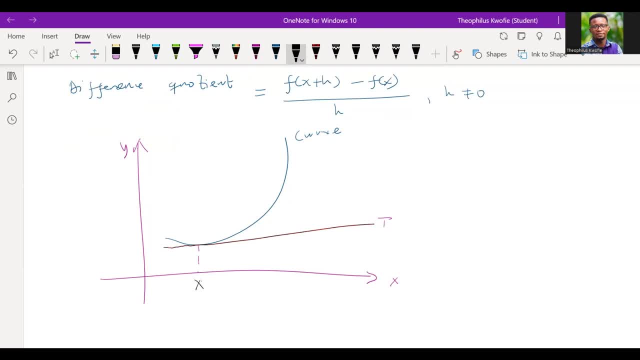 Let's call this point. Let's call it X, So the X value is okay. Now suppose that initially has gone through a change where we have X plus H, Remember H. I mentioned that it's just a small change that has okay to X, which means it. 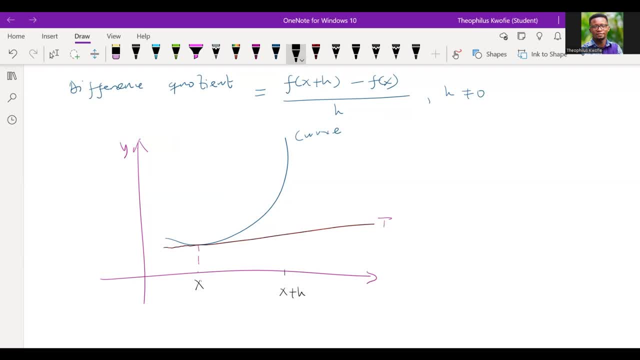 eventually shift the X value, right, Good Now. which means that we can find a, which means that At this point, okay, on the graph, we can find a value there. But the problem is that we want to stretch this curve. it's as if we are holding the. 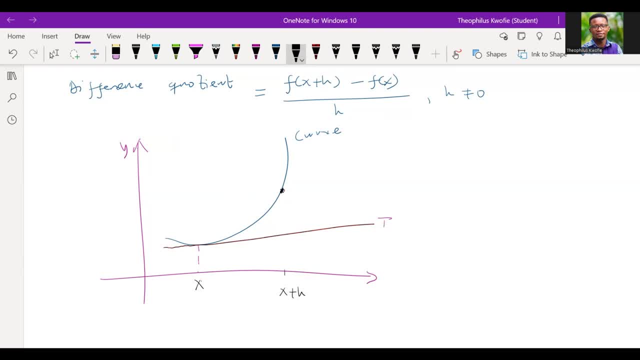 end point of the curve and trying to stretch it onto such a time or onto such a point, it lies on this tangential line. So this line is tangential in nature. okay, So a curve at a point is called a tangential line. 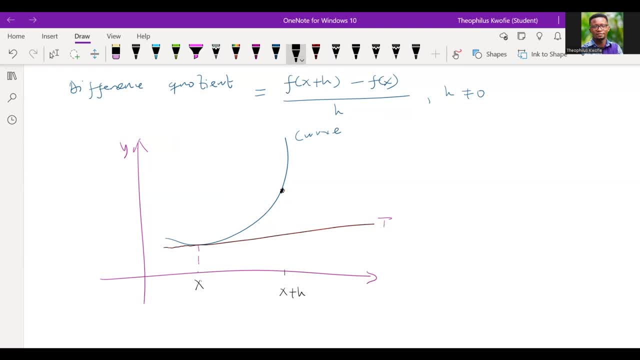 Okay, So a line that touches a curve at a point is called a tangential line. Okay, So let me write it a tangential line. Good, Now, as I mentioned, you want to hold the end point of the curve and try to stretch. 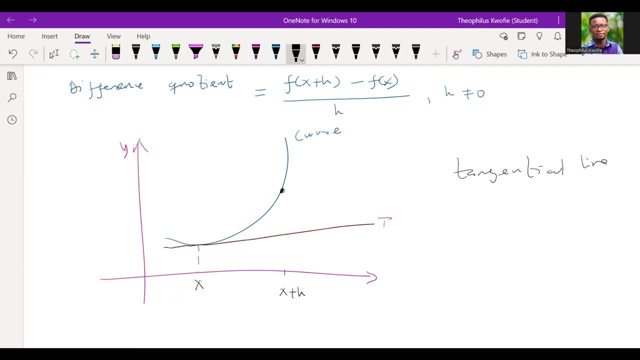 it onto such a time. it lies linearly on this line. What it means is that for us to do the stretching, what happens is that we have to decrease the H value. So let's decrease the H value. It means that we're going to have X plus H2 over here. 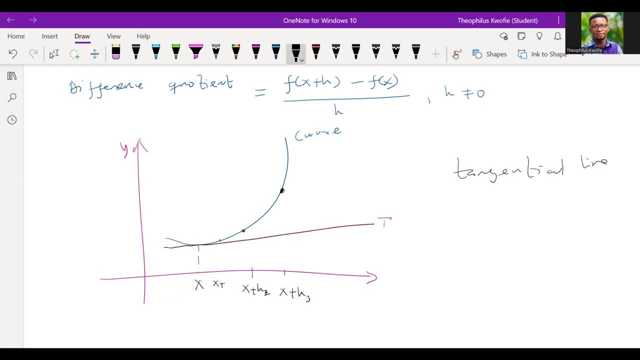 Then we decrease it further. Then we come here, We have X plus H. Then onto such a time we get to F, of onto such a time we get to the X point, Okay. So when that happens, it means that now, the distance over here, the distance over here. 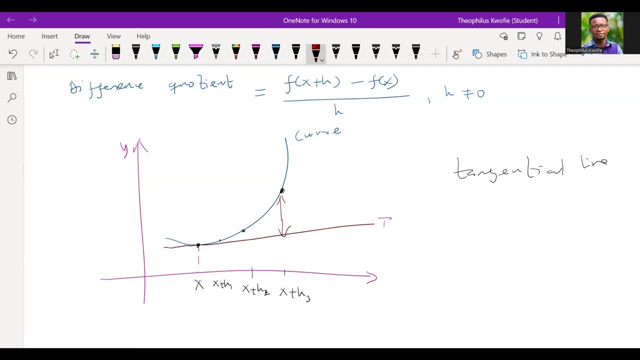 will now goes down right, The distance over here will now become very small, you know, very infinite. So the point we are going to make is that, as the curve is being stretched onto such a time it lies on this curve, you're going to have H value to H value to be very, very 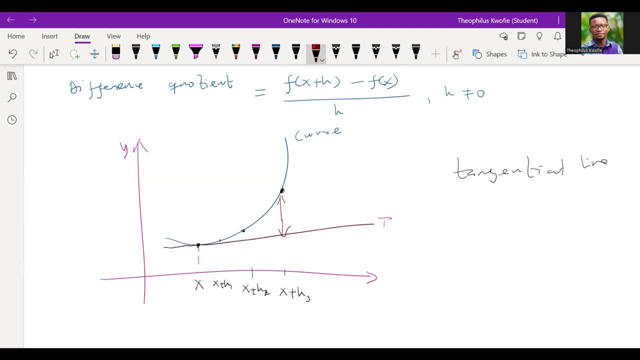 very small. Suppose that our initial H value, which is H3, was, let's say it was one, Okay, So until we get to H1, we will realize that H value would probably approach almost zero. Okay, So that is the notion over here. 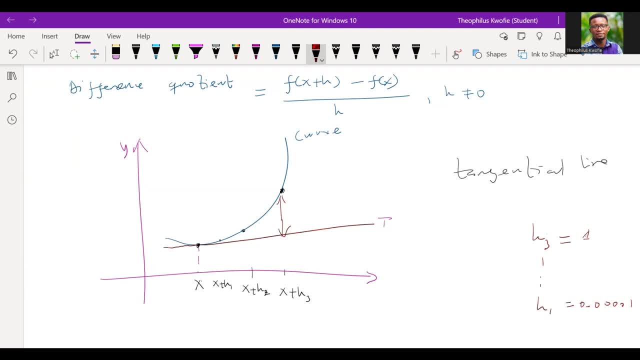 So we are seeing that the smaller the distance between- okay. we are seeing that the smaller the distance between the curve and the line- okay, the easier it is for us to solve the problem. That is what we are trying to do Now. having understood this, I want us to take this a bit further. 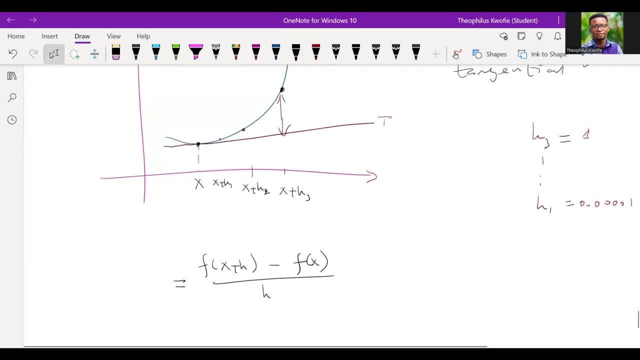 Now let's apply limit to the difference quotient. Okay, Now, already we know that difference quotient is being defined this way. Now, if we apply limit to the difference quotient as H approaches zero, what happens? What is happening? So it just means that we eventually become more or less like a line, right? 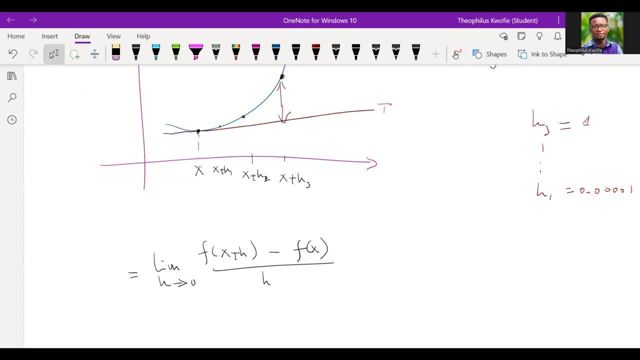 That becomes like a slope of that particular line. Do you all get it? So that becomes like a slope of that particular line? I hope we get it, So eventually this becomes more or less like a slope. So we call this one a slope. 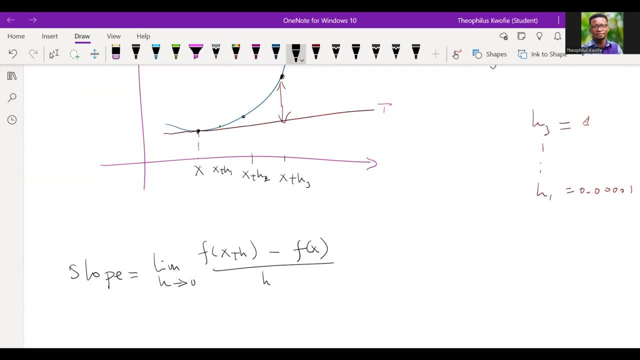 And I will also want to say that such a limit is also known as instantaneous rate of change of f, of x at x. So let's take note that this is also known as the instantaneous. This is also known as instantaneous. instantaneous rate of change of x, of f, of x at what? 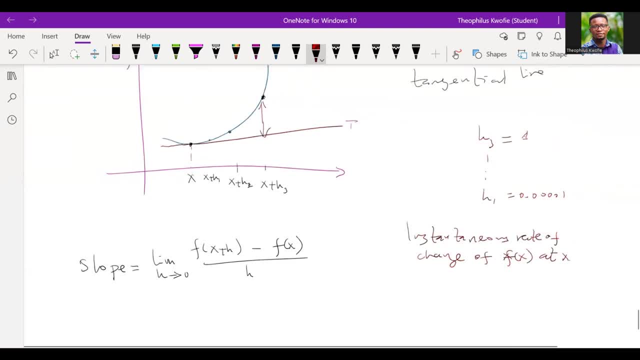 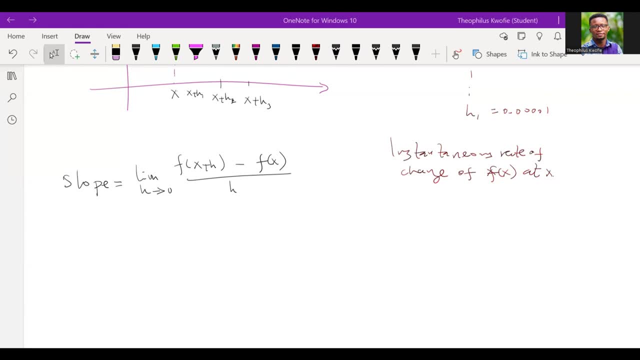 At x At x. Good, Good, Good, I hope we all get it. We said it's known as instantaneous rate of change of f of x at x. Good, I want us to now define it properly. Let's say, for a given function, for a given function, y equal to f of x. okay, then we 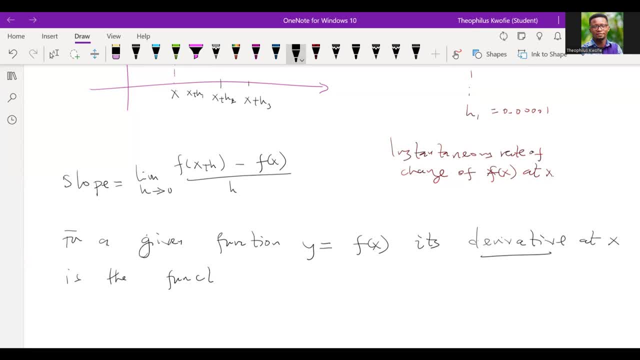 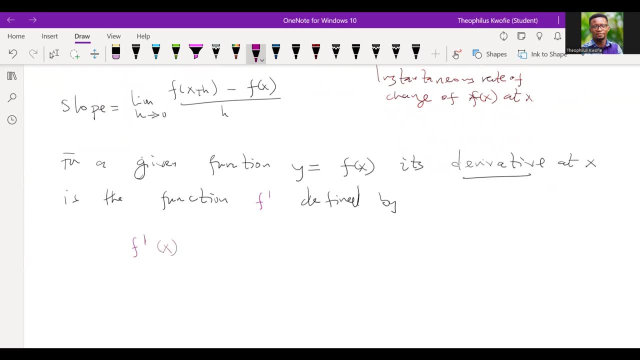 claim that derivative. we claim that a derivative at x is a function defined by, defined by f prime of x. So this is how we read it. We said f prime of x equal to the limit as x, h approaches zero of x, of f, the function being evaluated as these values. 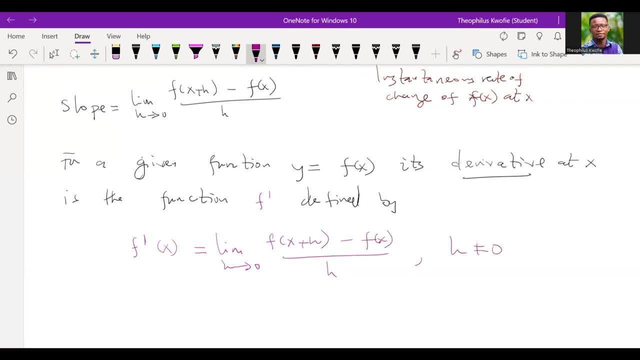 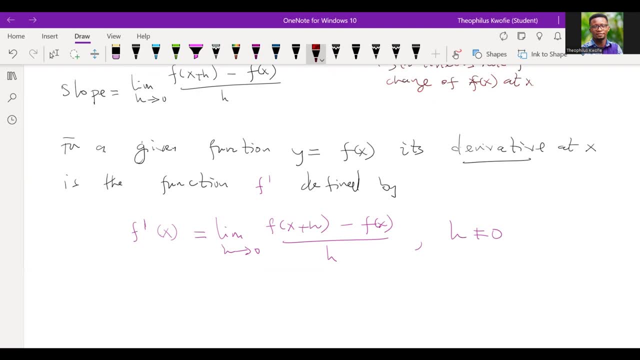 Okay. And we also said that h will never be zero, provided that the limit exists. So let me say that, provided that the limit exists, Okay. I would also want to kind of state that if f, prime of x exists, then we say that that. 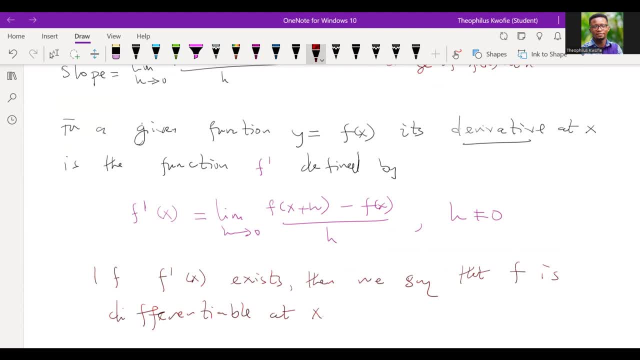 if f prime of x exists, then we claim that f is differential at x. So let's take note. Now I want us to look at the function. Okay, Let's look at the first example. So let's go to the first example of the day. 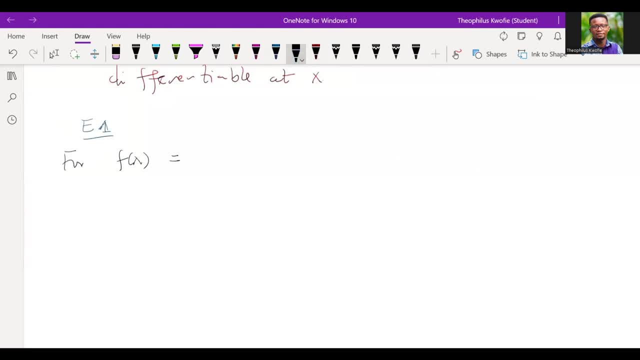 So with example one. So for f of x equal to x squared, Now find f prime of x using the limit definition. So what is the limit definition? We claim that the limit definition. so f prime of x will be equal to what? 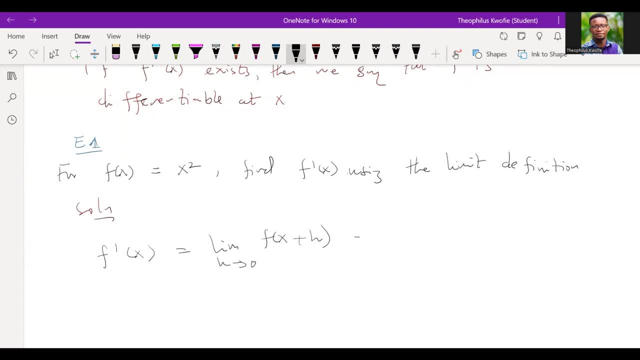 Limit as h approaches zero of x plus h minus f of x, all divided by h. But then we claim that h should never be zero. Good, So how do we solve this? How do we continue with this? Now? what we'll do is that. 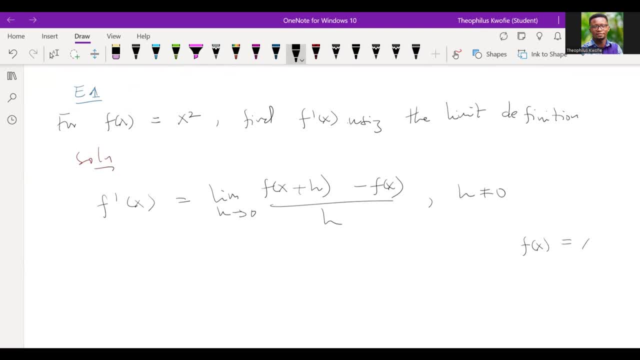 So if I have f of x will be x squared. then it means that if I want to find f x plus h, it just means that wherever I see x, I should replace it by what X plus h. We looked at that last week. 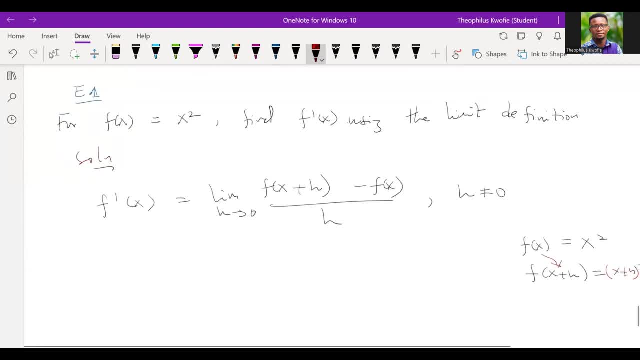 Okay, So that means that wherever you see x, we just replace it by x plus h. So we employ the same thing here. So let's go. So wherever we see x, we replace it by x plus h in the main function. 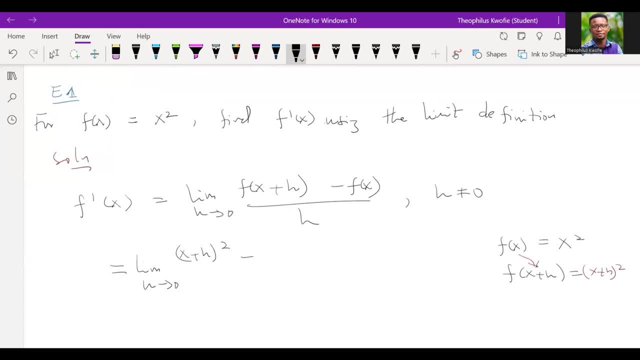 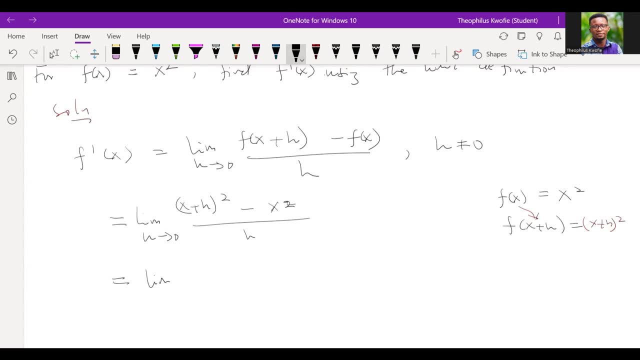 And that gives us what X plus h, all to the power two minus f of x. But the question is: x squared? Now, when we simplify the numerator, when we expand and simplify, we should have x squared plus two, x plus h squared minus what. 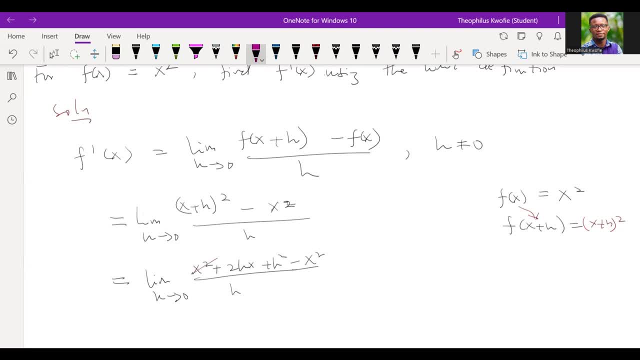 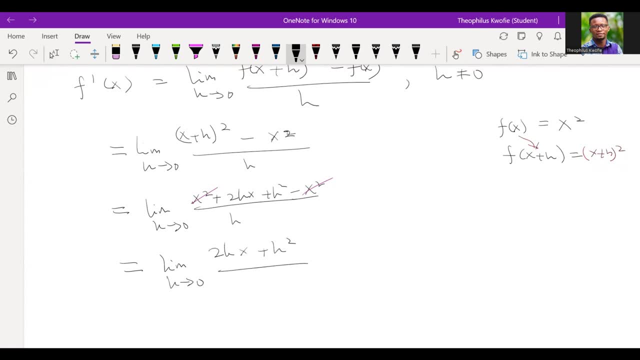 Minus x squared. So when we look at it, we can do some cancellations, right? When that happens, we're going to have limit, as h approaches zero, of two x plus h squared all divided by that. But this can't be simplified, right? 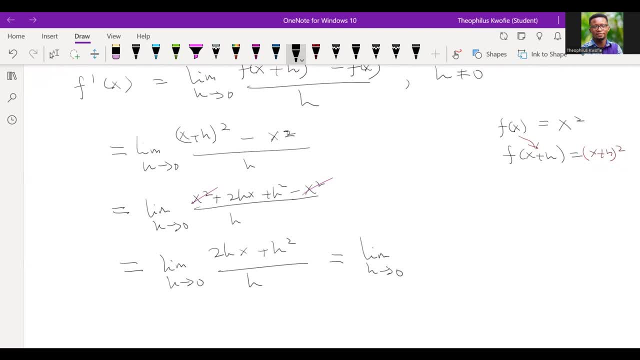 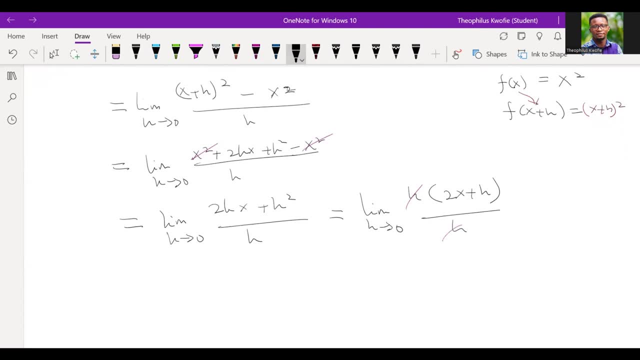 So, which means you're going to have limit as h approaches zero. When you factorize the h out, we should have two x plus h, all divided by h, right, And this is that So, in which case we should have limit as h approaches zero of two x plus h. 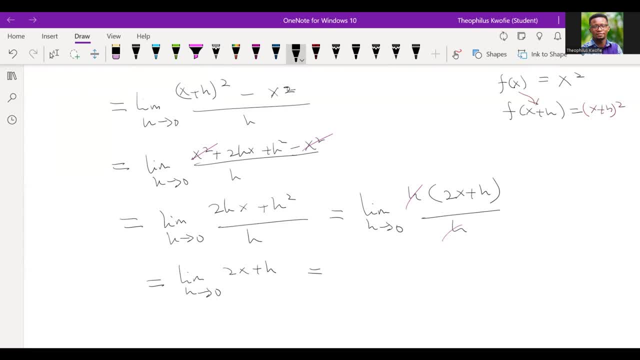 Now, this is where we also employ one of the laws of limits. So what this? what is straight away? what it means is that wherever you see h, we should just replace it by all zero right Plus a simple function. Okay. 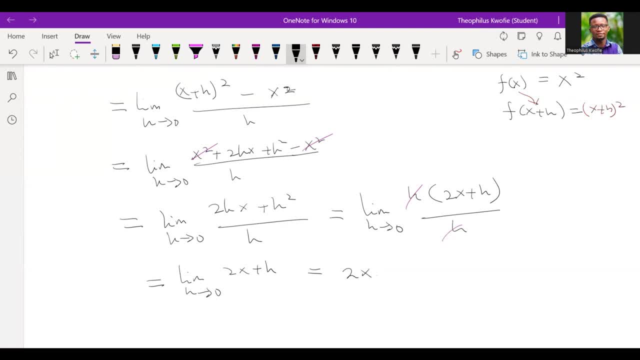 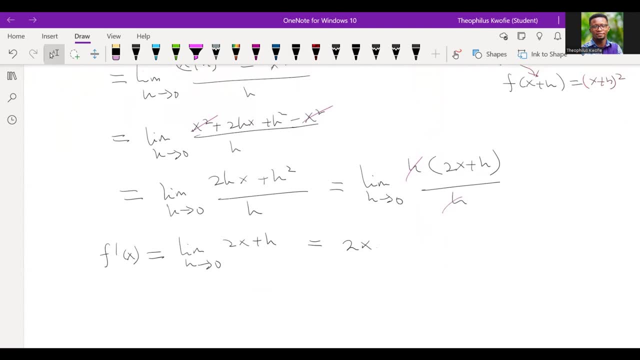 So we just plug it there We have. So it means that any time we differentiate a function x squared, its derivative is two x or its slope is two x. Okay, So derivative is also known as the slope, as we saw that in our illustration. 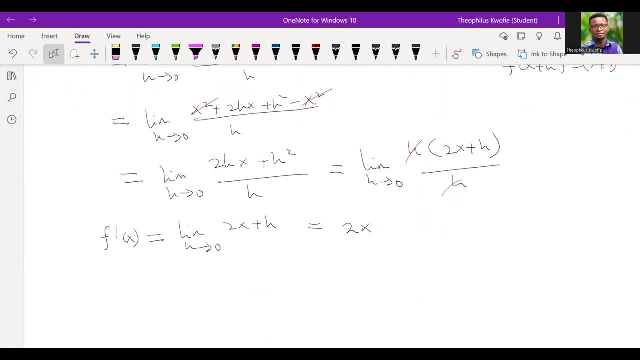 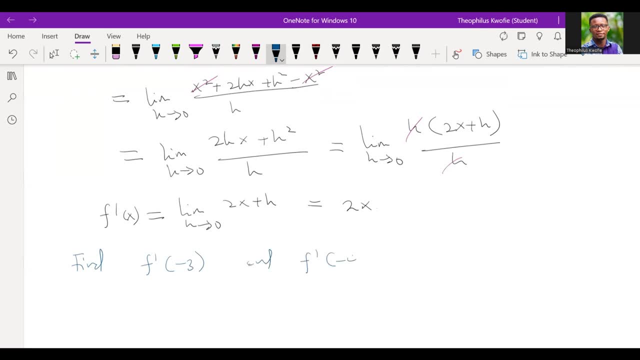 So I want us to take notes. Okay, good, Now find this. What if I want to find f prime of minus three and f prime of minus four, The differentiator function being evaluated on negative three and that of negative four? Okay, 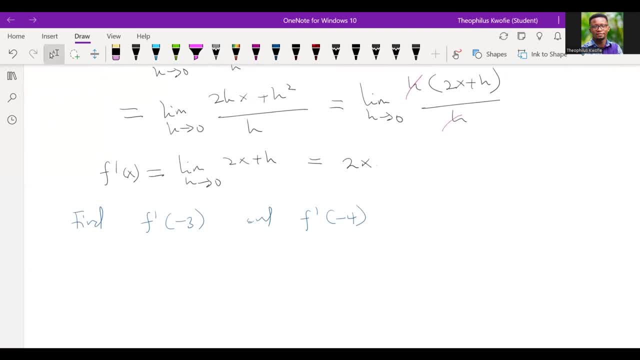 So when that happens, it means that wherever I see x in the f prime of x, as you just replace it by minus three, right? So we have f prime of x being equal to two x. So now, what is f? prime of f, of the of the differentiation function being evaluated on negative three? 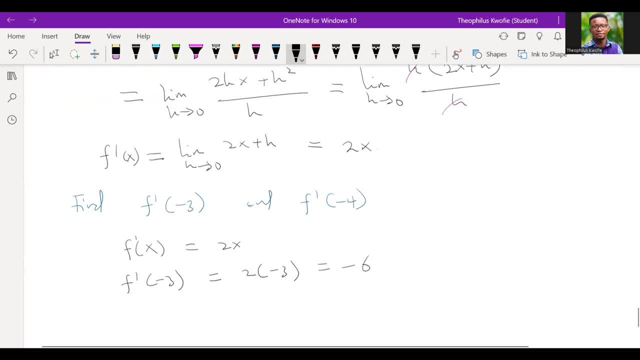 It means that I will have something like this: So you can do the same for the second pattern, Right. You can do the same for the function being evaluated on negative four. So let's look at so. with example two, let's look at a situation. 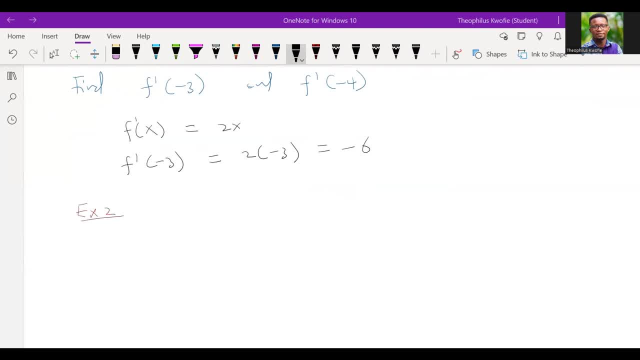 Now I want us to look at it. What if that? what if that decimal round, my f of x, is a cubic function? How do I find f, prime of x using the limit definition? So we go through the same procedure, Okay, good. 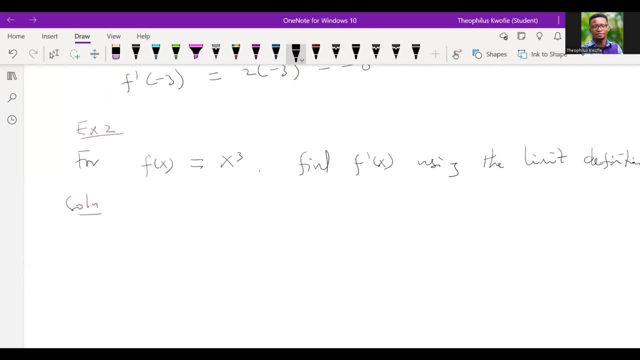 So if I have such a function, then it means that, by using the limit definition, f, prime of x would just be equal to the limit As h approaches: zero of f of x plus h minus f of x, all divided by h. So using the same principle, which means that we, by simplifying, we should have something. 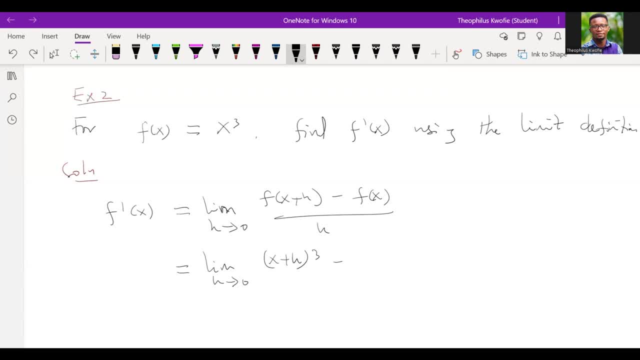 like x plus h to the power three, minus what S to the power three, all divided by h. right Now. last time we kind of solved a similar example, so I would go straight to the point Now by simplifying the expression. 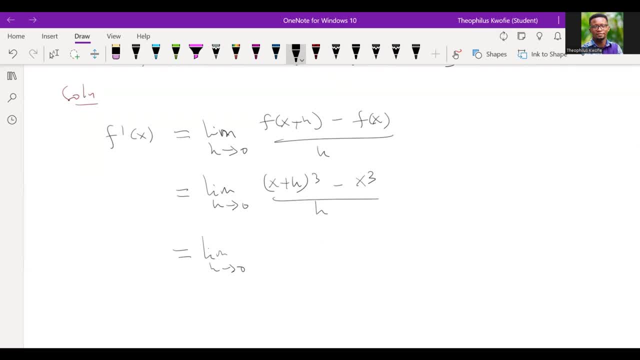 under the, under the cube, something that when we expand, we should have. something as this. so i explained the last time. so i wanted, if you have any any problem with this, you want, to visit the previous content and i think you will be able to, so to get it. then we can simplify this a bit and 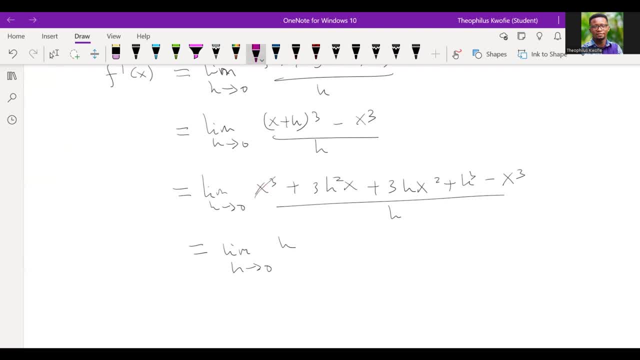 that should give us what we can pull out: the h over here we can do some cancellation. then we kind of pull out the h out and when h is pulled out we should have some as this: right at this point we can still do some cancellation, which means that we're going to. we said that the limit 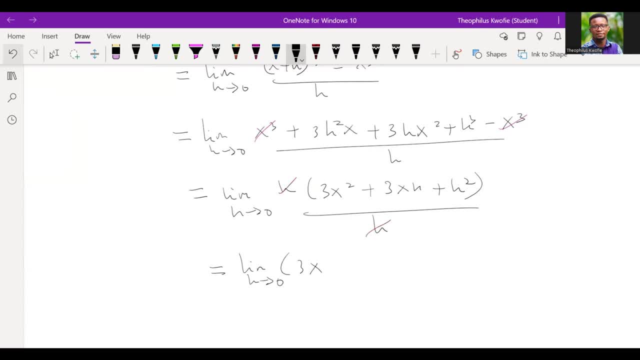 of a sum. we claim that. remember this: what we said, that the limit of the sum as one of the laws of of limit. we said that the limit of the sum is the word is a sum of the limit. so take notes, all right. so when we plug in it wherever you see, wherever you see h, we should just plug in um zero now. 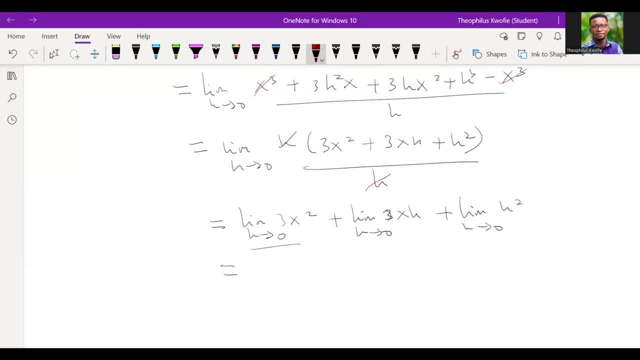 when we plug in now over here in the first function, we don't see h there. what it means is that: um, This is just a constant. If h is not found here and this just means that h is this 3x squared. it's just a constant. 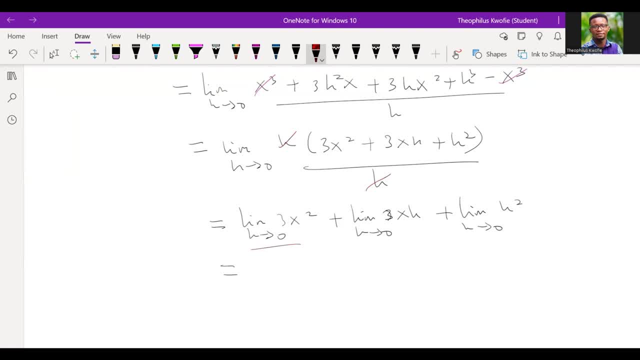 And we said that at the limit of a constant. we said it's a constant right. So this means that over here we should have 3x squared right, And over here, when you plug in here, it runs to zero because h is zero here. 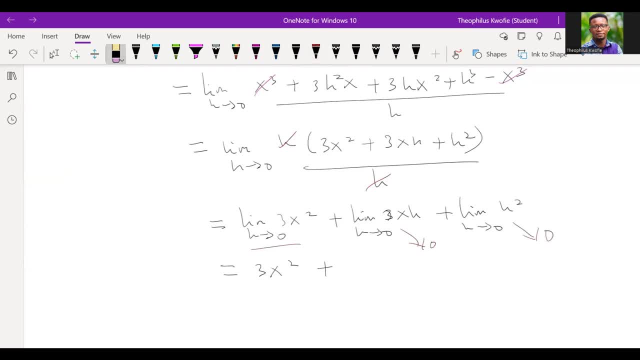 Also, h runs to zero. okay, So in that case, we're going to have only 3x squared, which means that anytime we differentiate x to the power cube, we should have 3x squared. okay, Good, good, good. 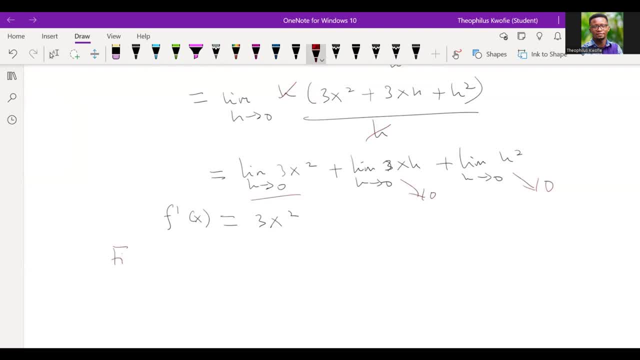 I believe we are all getting it. So if I, everybody, if I- was to find f prime being evaluated at one, what it means is that? so this implies that wherever I see x, I should just replace it by one. okay. 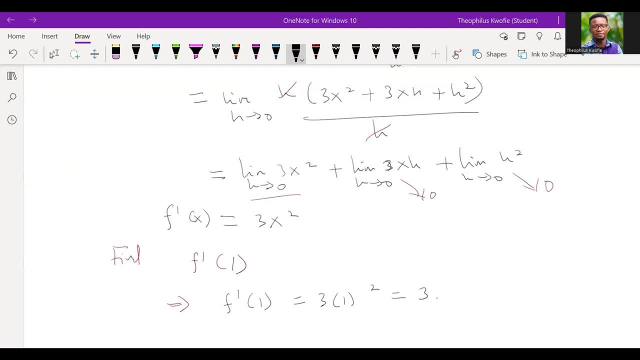 And that gives us something like this: I believe we are all getting it. Are we following? Good, If you have any questions, please put it in the comment section and I would inspect it. So I want us to solve one more example, okay. 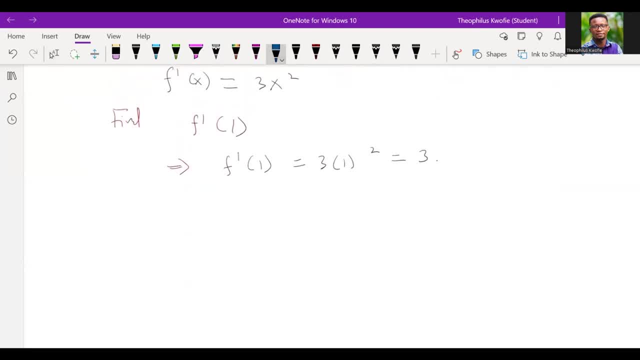 I want us to solve one more example. Then we kind of look at other interesting stuff. If I give you f prime of x and then the b, you want to find f prime being evaluated at two, Then the c part. I want us to find an equation of the tangent line. 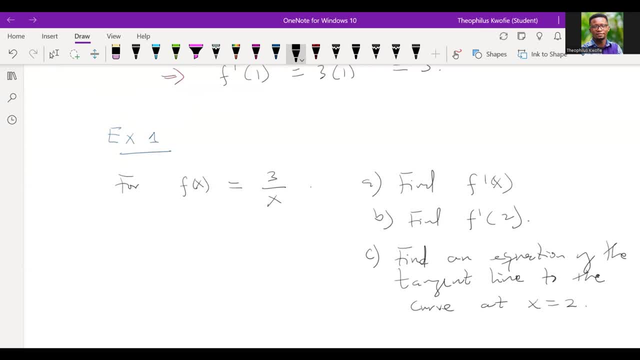 to the curve at x equal to two. So at this point I want you to pause the video and attempt this question. All right, So I believe you have your result. So let's see what we can, what we are going to get. 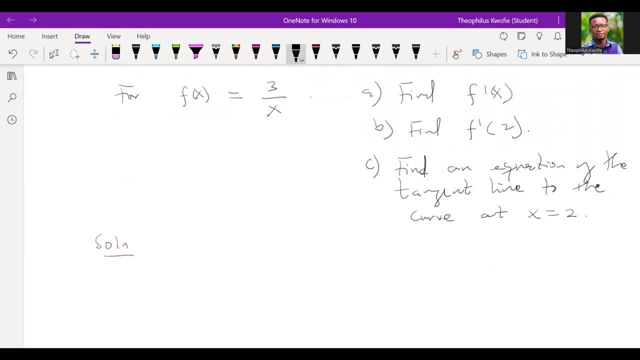 Now that you have your result, Now I'll pay your result to what we have here. All right, So we have f of x being equal to three, all divided by x. Now, using the limit definition, it means that f prime of x. 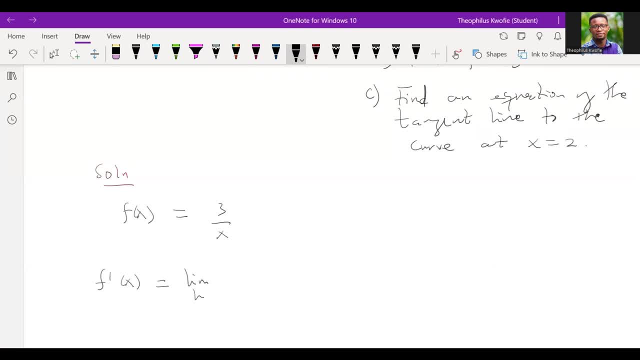 which is also known as the slope, is equal to limit, being limit as h approaches zero of f x plus h minus f of x divided by h. But then we said that h should never be zero. All right, Now what we do is that wherever we see x, 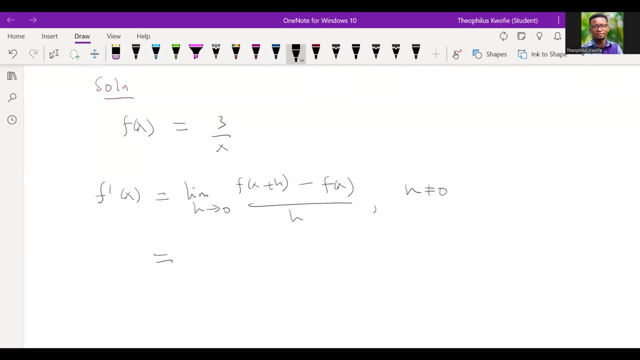 we just replace it by: in the first case, we have f x plus f of x plus h. Okay, So in that case you should have something like this: And then for f of x, already we know the value of f of x. 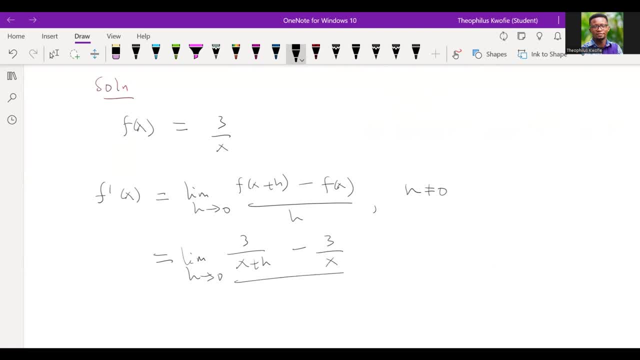 Okay, We know the function. So that is our array on x all divided by h. Okay, So let's take note Now. it just means that over here we just have to simplify. And when we simplify this, what do we get? 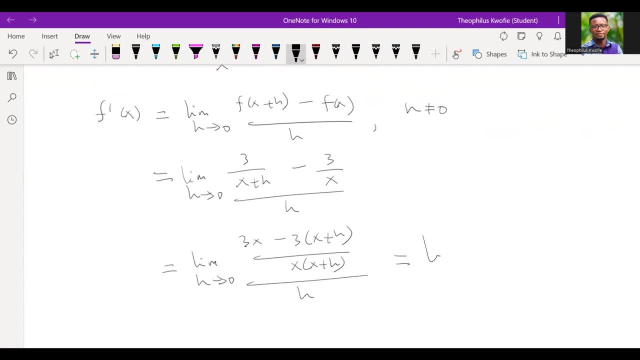 We should have something like this: all divided by h. Then, when we go further, to simplify this, we should have all divided by h. Okay, Now let's simplify this a bit, And when we simplify this a bit, we should: 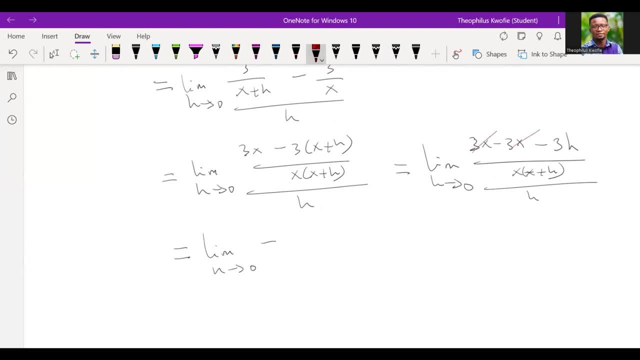 because over here there'll be some cancellations, So we shouldn't be able to have something like this Now. now all divided by h, But last week we- I- explained something, So this will cancel this by um algebraic manipulation. 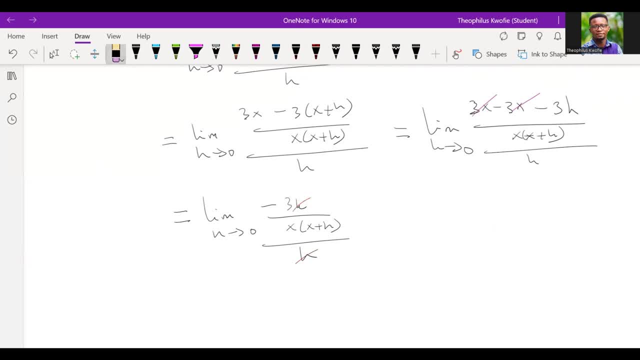 We claim that a divided by b- let me use a different pencil- So a divided by b divided by c. Okay, Can be written as this: We, we said that we can reciprocate the c and that gives us what one over c. 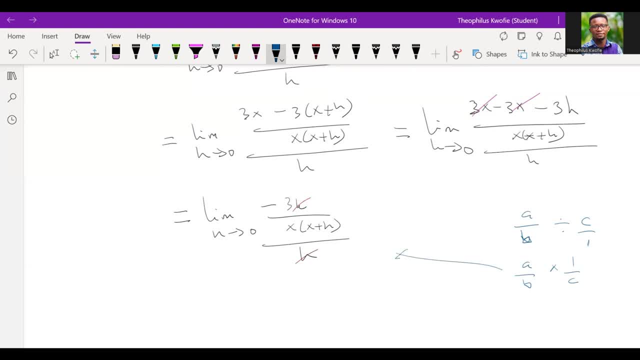 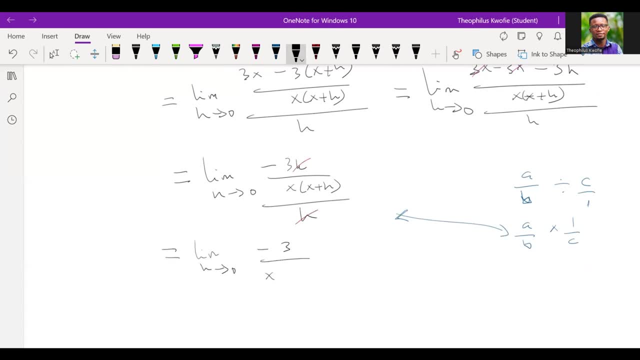 So it's the same thing over here. So when you apply the same thing here, you should get that Okay, good, So let's take notes. So when that happens, you should have limit. as h approaches zero of minus three on x. 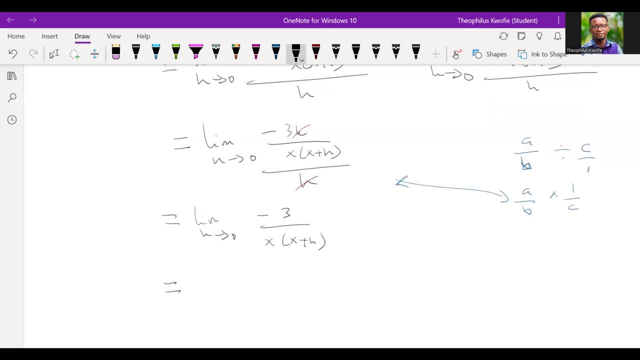 x plus h. Now what did we say? This is in the previous episode. we said that the limit of a quotient is a. what Is a quotient of the limit? So the limit of the quotient is a quotient of the limit. So take notes. 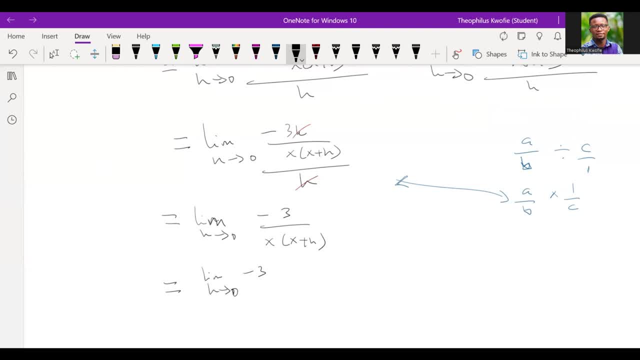 So now, what is the limit? The limit of the function minus three over the limit, as h approaches zero, of x plus x plus h. Now, what is the limit of minus three? The limit of a constant, we said, is a what It's a constant. 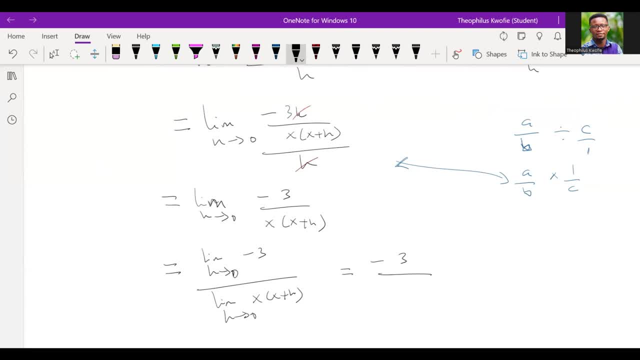 right. So the limit of a constant is a constant And when you look at a denominator, it just means that wherever you see h just replaced by zero- and that happens- you should have something like what X squared. Let's take note. 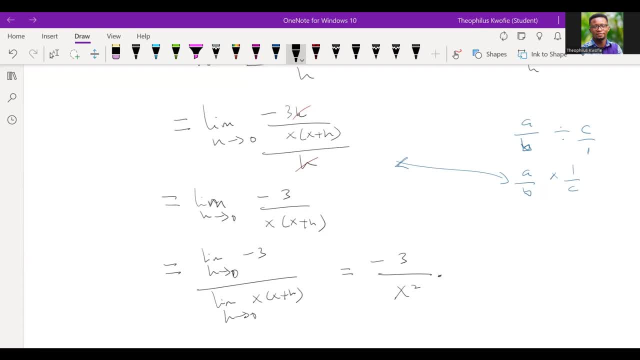 So when we simplify this, we should have something as this: Okay, For the first derivative, you should have something as this. Now let's put a big part of the problem. The big part of the problem says that we should evaluate the differentiated function at two. 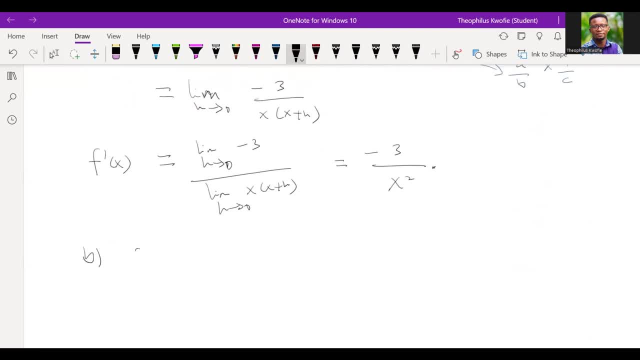 Okay, So that's the big part. The big part says that you should evaluate the differentiated function at two, So which means that wherever I see x, I should place it by two, and that should give us what minus three on four. Now see the c part. 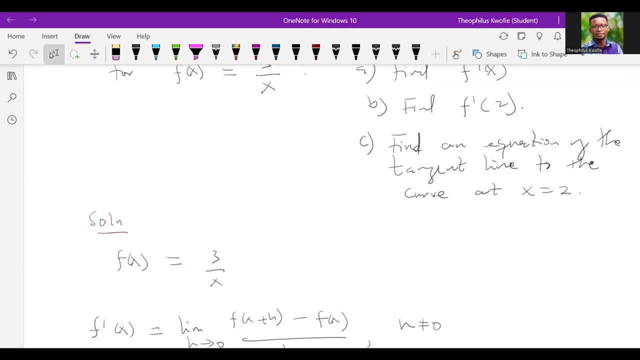 the c part, we are told to find an equation of the tangent line to the curve at x equal to two. Find an equation of the tangent line to the curve at x equal to two. So this is a very interesting question. I believe that it's in every year. 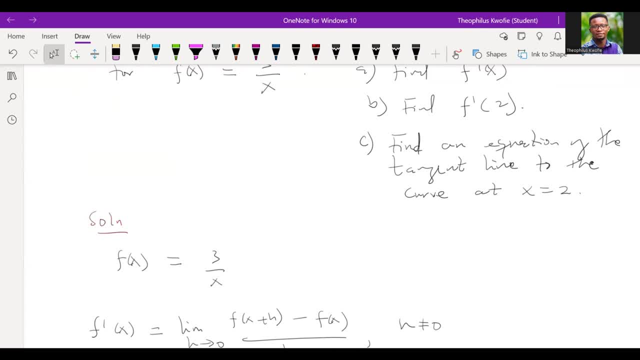 This is the kind of questions I give to my students And sometimes when they when they see questions like that, they fumble, because it requires that you know the difference question. It requires that you know how best to find certain things before you attempt this question. 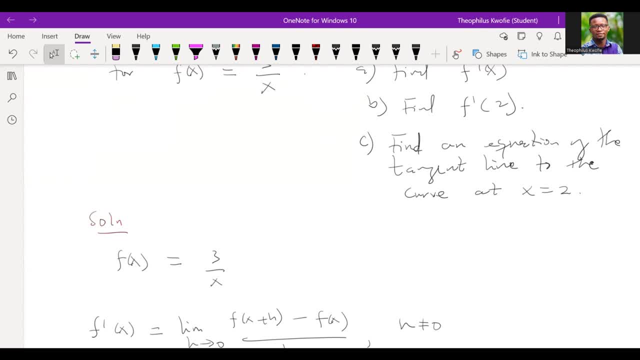 So if you don't know how to find the first problem, it means that you may not be able to attempt this. So this is an approach, This is an opportunity for us to learn something that we can hold on to any time we are called on to produce the results. 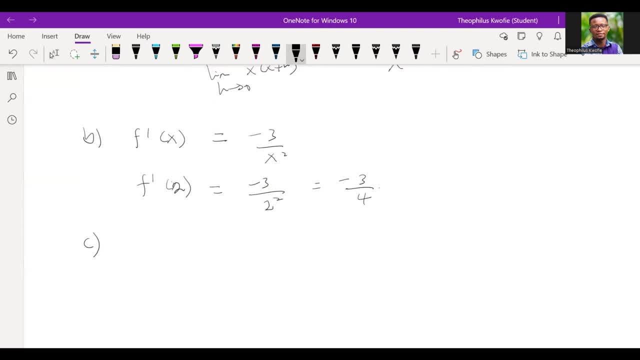 So I want us to take note. All right, So for c now. we said something about the tangent, the tangent line. So the tangent line is just like the normal sample line. The normal is y equal to mx plus c, and the m is known as what? 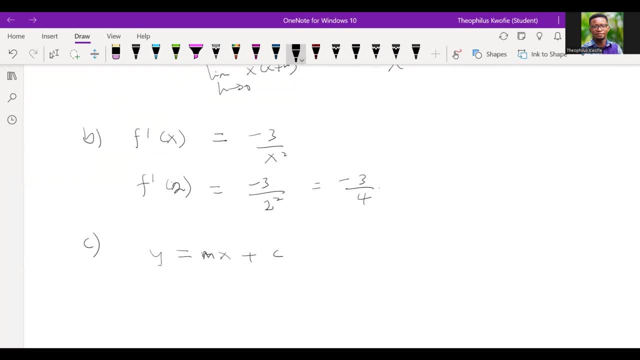 The slope And the c is just the what we call the y-intercept. Okay, So let's take note. All right, So we already been kind of. we know our m. what's m is a slope. It has already been evaluated. 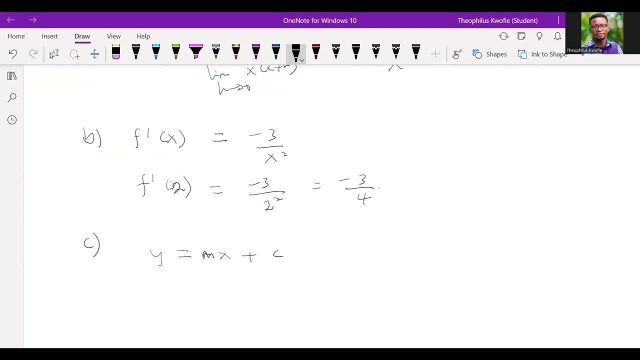 which is what minus three four. Okay, So our m, already we know. our m is what we call the f prime. Okay, The f prime is also known as the slope, Our m, already we know, which is already been evaluated at negative three. 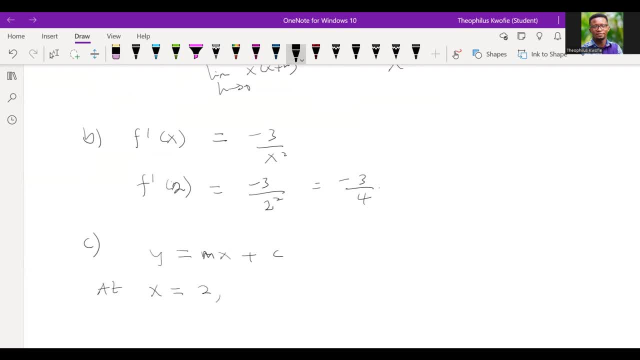 So at let me state that x equal to two, Our m is equal to what Minus three on four. So let's take note. Now. it means that we have to find our y. Okay, How do we find our y If you know your x? 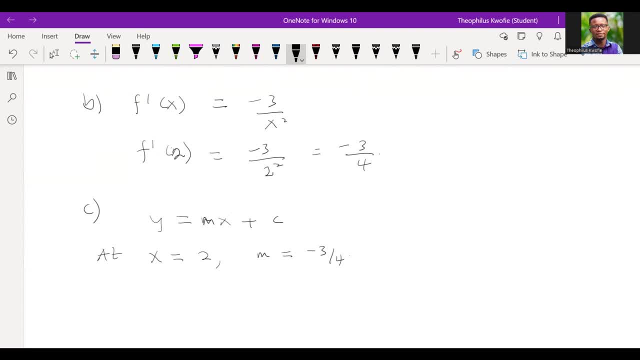 how do you find y? So already we know the main function. So our y is also the same as this right. Our y is also defined as what f of x? Our y is the main function. So if it implies that our y should be equal to f, being evaluated at two, 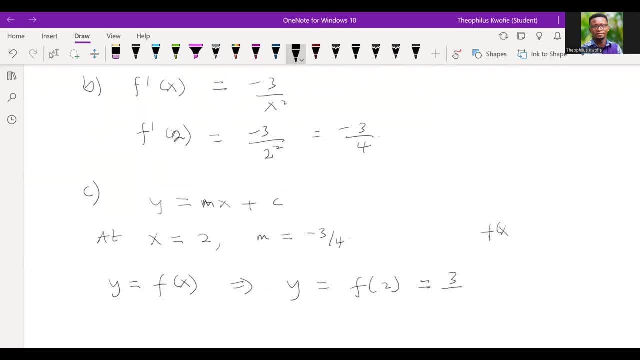 But what's our main function? was what main function? Let me write it here Also: three on x: Okay, So now, if you evaluate it, if you evaluate this function at two, we should have something like this right now, The point of this: 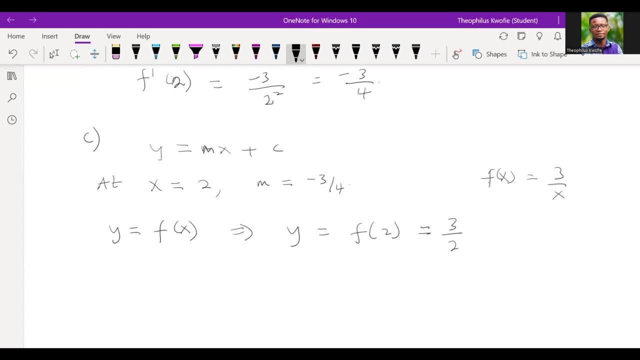 I mean, the whole point is to try to find c. Okay, good, Now we have to plug all of this back into into this equation. Okay, So now, by plugging in into the into the main equation, we should have something like three on two equals. 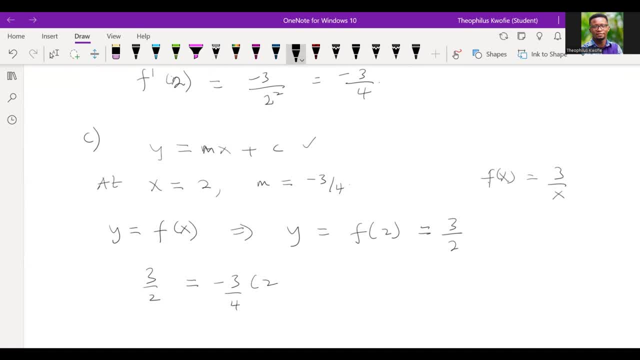 What's our m? We know is this: What's our x? Our x is two. Now this will help us to find our c. I hope we are all getting it Now. when we simplify, you should have c to be equal to what. 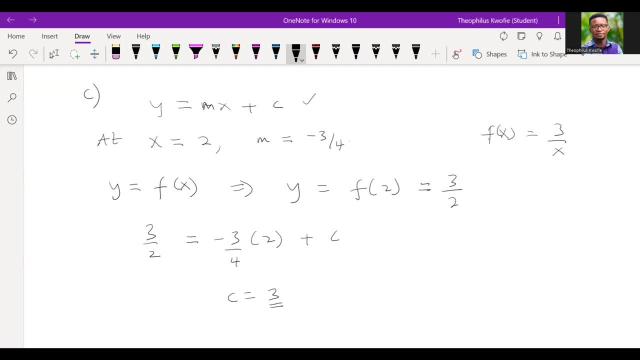 Who can guess the answer for c? Our c should be what? Should be three Good When you simplify. our c should be three Good Now when you plug it back. So this implies that mine should be what, Because now we know our m. 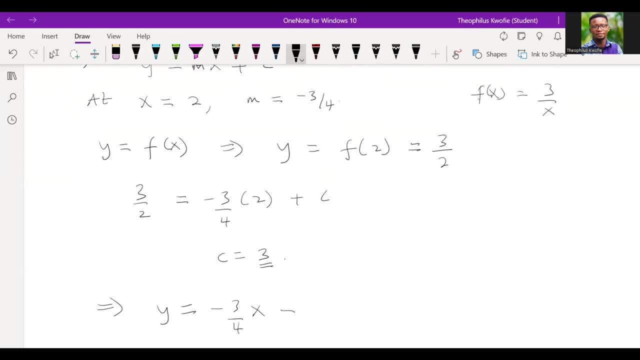 Should be what Minus three on four x plus c, Our c is what Three. So this is the line to the curve at, this is a tangent line to the curve at m. Okay, So now we have m x equal to two. 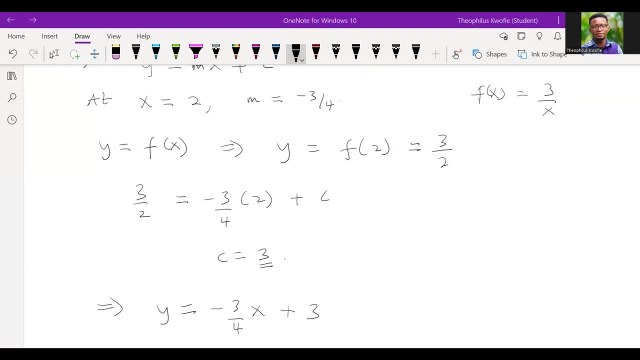 So let's take notes. I hope at this point we are, we are getting it right. This is a spot. I would want to kind of emphasize that This is an interesting section, but I believe you will not want to miss. It is very interesting. 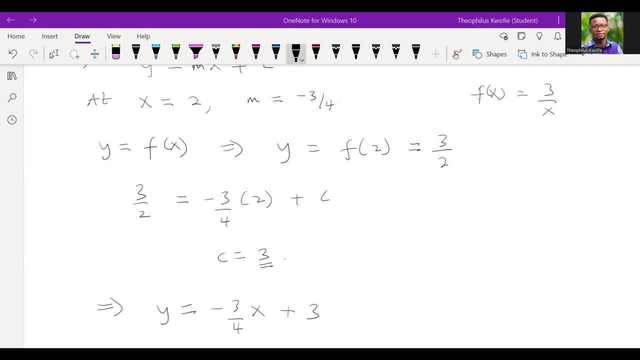 You may want to understand all of these things, but these are applicable to a real world situations And I would at some point. I will bring in an example that is, that is relatable. Okay, So please take notes, Even as we. 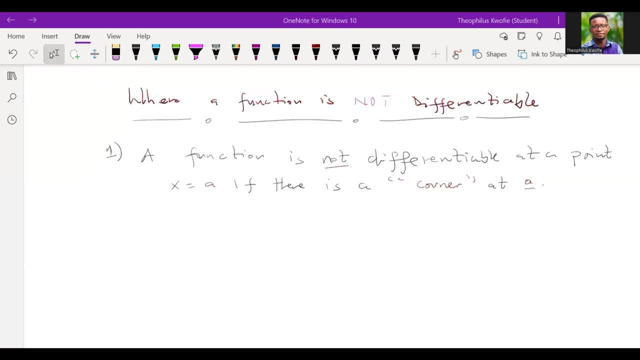 as we explore, say, journey. now, at this point, I want us to look at a very interesting thing Now. is there a function that is not differentiable? Is there a point in a function say that it's not different, or that situation? Are there some situations? 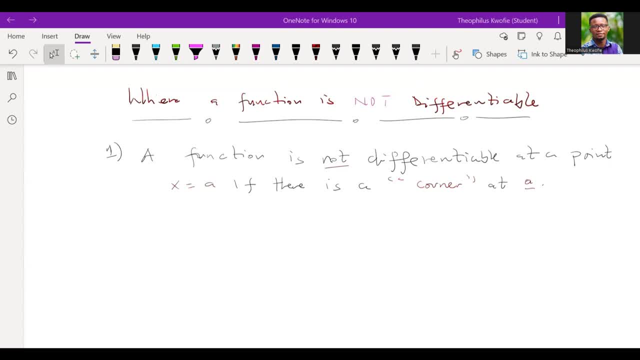 you know where a function may not be, So that is when I just point us to look at it. Okay, Now, one of the first condition for which a function may not be differentiable is this: If there is a corner, okay, 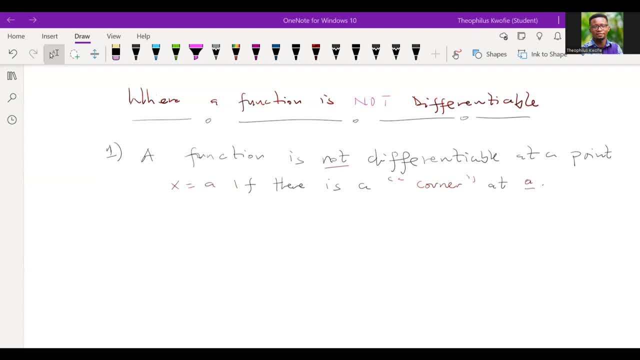 If there's, there's, there's, um, there's that what you call a caps. If there's a caps or a corner in a curve, it just means, or in a function, it just means that such a function is not differentiable at that point. 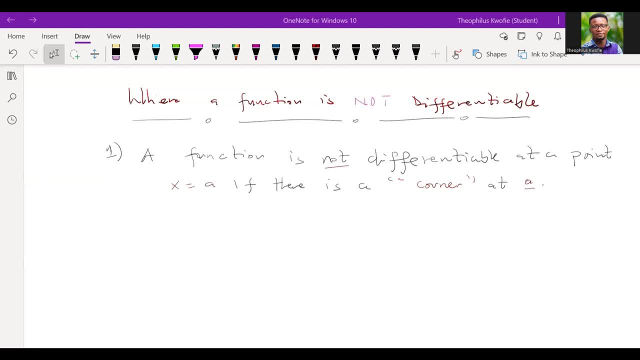 So I want us to take note If there's a corner or what we call caps. okay, If there's a corner or what you call caps, it means that the function may not be differentiable at that particular point. So let me do some few drawings. 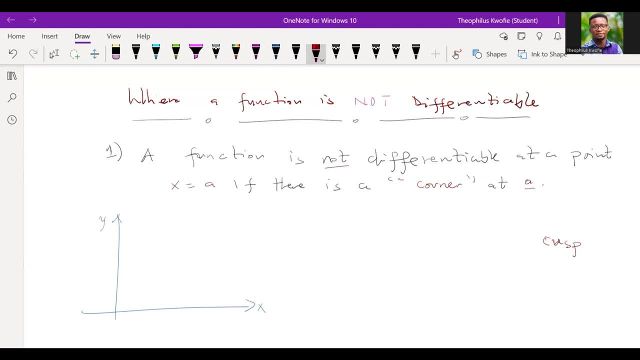 Um, so let's look at a curve as this. So I have something as this: and A is defined here. Now, over here, for example, when you trace the A down because this is a corner, we claim that A will not be differentiable at this point. 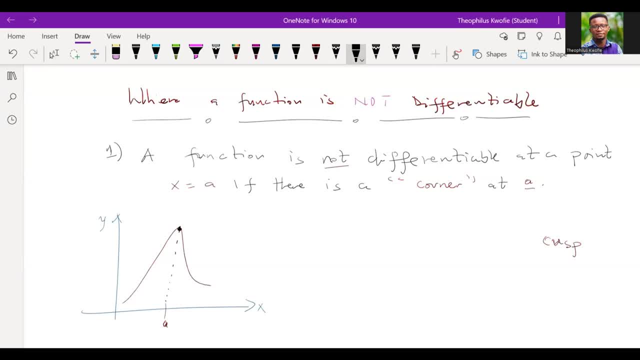 A will not be differentiable at this point. Sorry, The function will not be differentiable at A. How are we getting it? If we have a curve like this, it's just because there's a corner here or a caps over here. 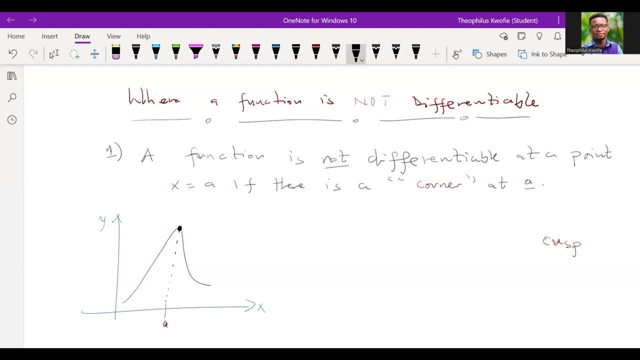 it just means that the function will not be differentiable at the point A. So let's take note. Another example is a function, a graph, as this, So let me define it this way. So I have a curve as this, then something as this: 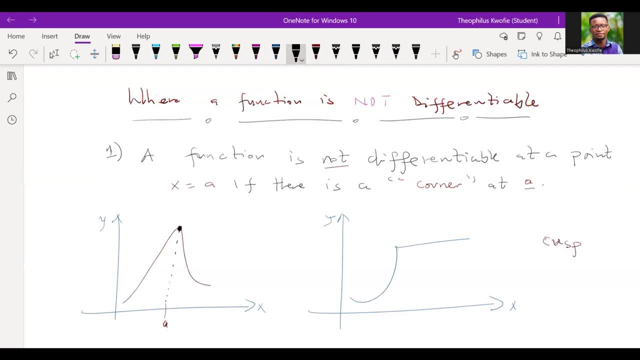 Over here we claim that if, for the instance, if I trace it down here- it just means that A will not be differentiable at this, such as such a point- Okay, Because this point is a corner. it just means that A- just made a function- will not be different at the point A. 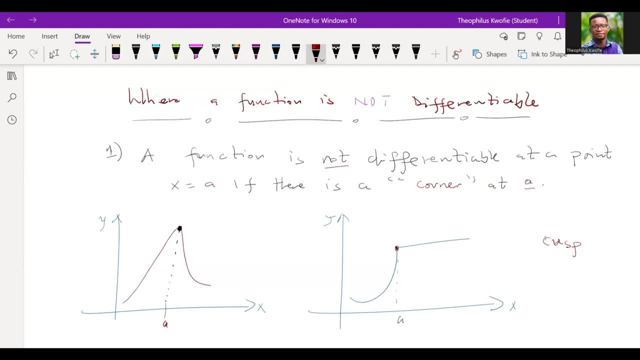 Are we all getting it Good? So I want us to take note that if, for as long as there's a corner, or some corner, or what you call a caps, it just means that the function will not be differentiable at the point A. 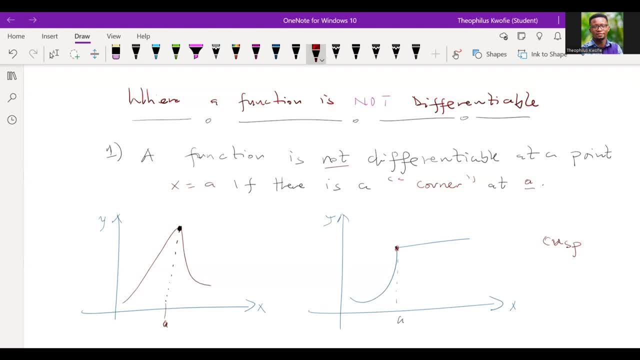 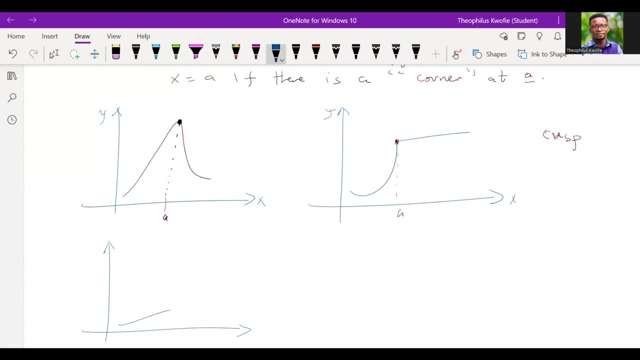 It just means that the function will not be differentiable at the point A. It just means that the function will not be differentiable at that point. So let's take note And that last example, also the last example for the last ration, will be a graph as this: 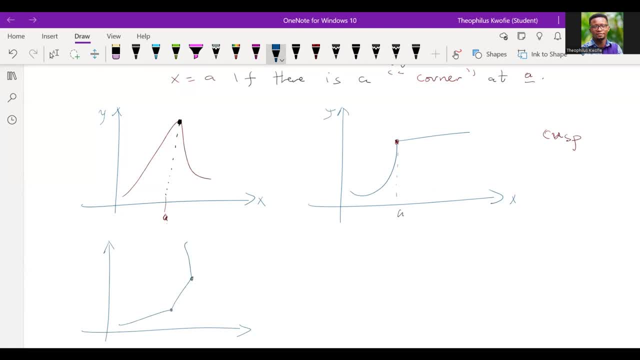 And I come this way. I have a point here, I have another point here. So the graph will not be differentiable at A1.. Also, the function will not be differentiable at A2, because these are all caps. So let's take note. 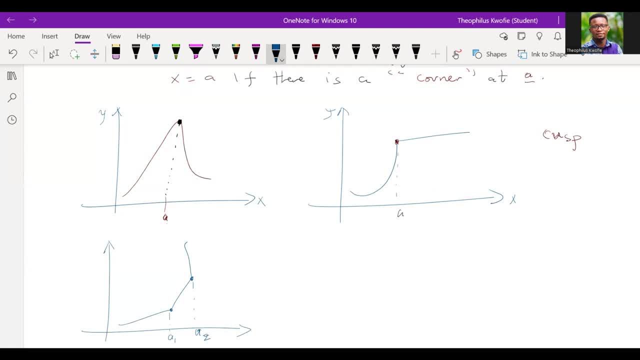 These are very interesting things that I believe that they are crucial and you don't want to miss them. If you have studied calculus and you do not know this, it means that there's a loophole that you have to fill, And these are some of the things that you don't want to miss. 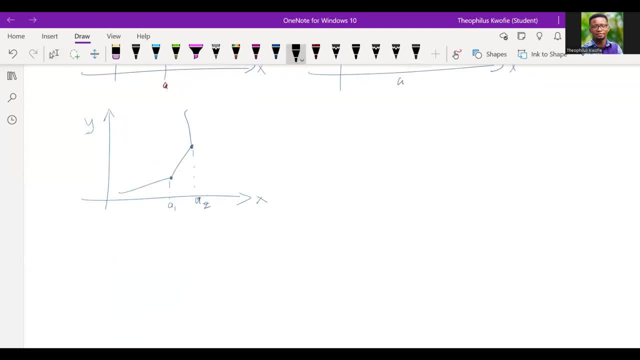 It's very, very important. So please, let's take note. Another condition that I want us to consider is when there's a vertical tangent at A. So I'll write that a function f of x is not differentiable at a point x equal to A if they have a vertical line. So I'll write that a function f of x is not differentiable at a point x equal to A if they have a vertical line. So I'll write that a function f of x is not differentiable at a point x equal to A if they have a vertical line. 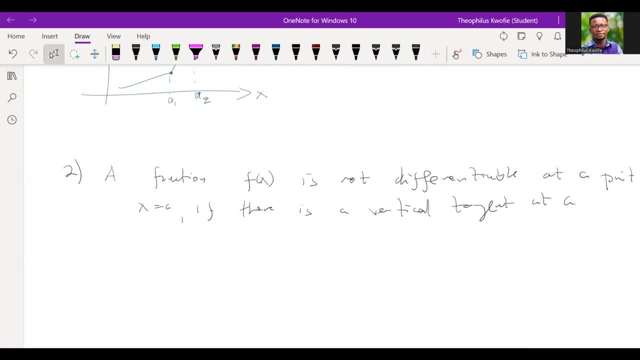 If there's a vertical tangent at A. So let's take note, please. Let's take note. So if I have a graph as this, let me see if I'll be able to give a simple graph. I have something like this: 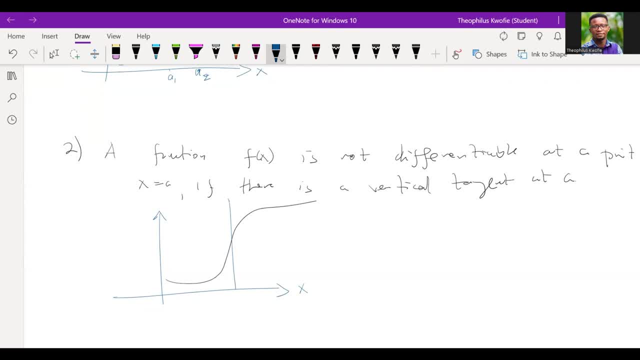 Okay, Then I have a tangent line as this, Such that I have a tangent that passes through such a point: We claim that such a graph or such a function, the graph of that function, will not be differentiable at a point A. So I want us to take note. 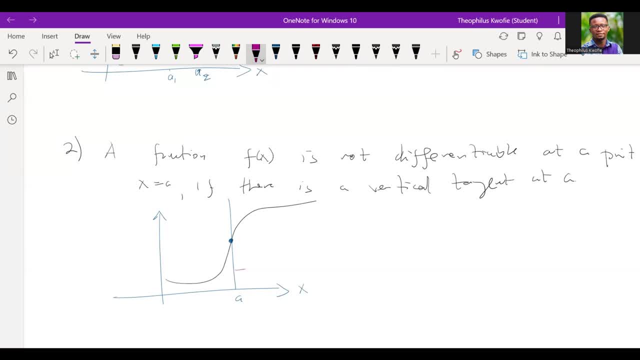 Okay, That's very, very important. So this is a very, very important Vertical line. Okay, So, this is the vertical line. Okay, So we claim that such a graph would not be differentiable at a point. So, please, I want us to take note. 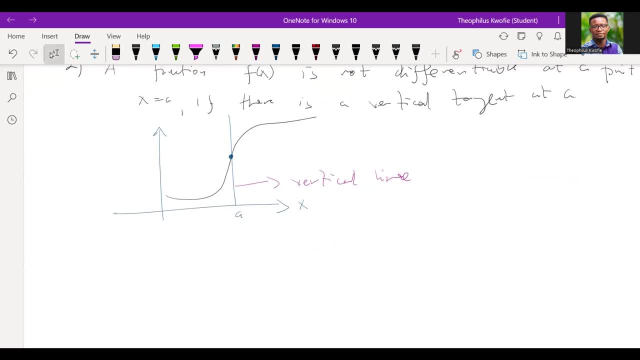 Please, let's take note. And then the last condition that I want us to consider is that a function is not differentiable at a point. x equal to s equal to A. A function is not differentiable if it's not continuous. Okay, 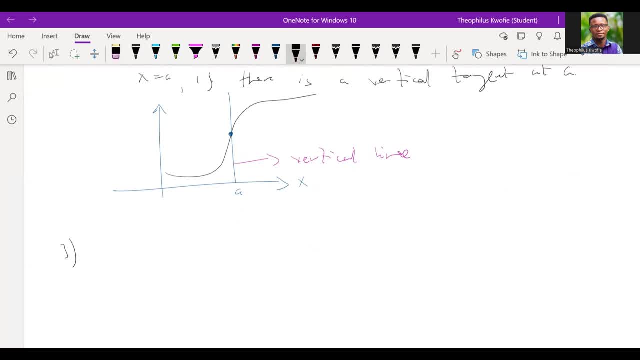 So let me write it down for you guys That a function f of x- okay- is not differentiable at a point x, At a point x equal to A, if it is not continuous Okay, Let me stress on this that if it's not continuous at. so let's take note please. 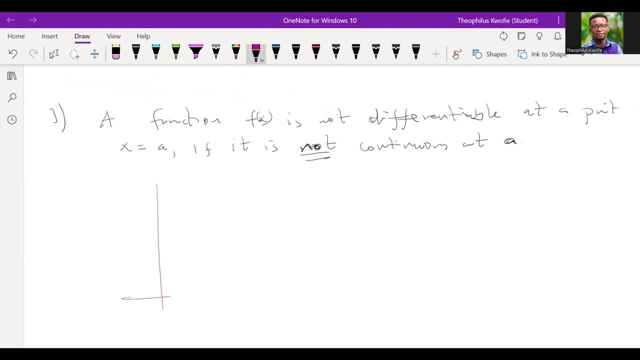 All right, So let me give a graph for you, for me, for us to understand this. So if I give you a graph as this, I think this graph is not that interesting. Let me give you this graph, Let's give it. give a graph as this: 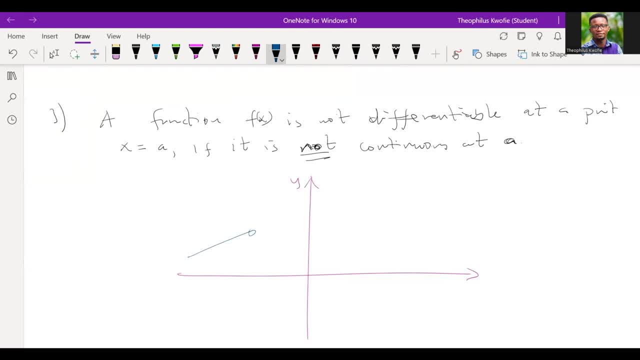 So if I have this graph, let me bring another graph. I kind of use this. So this is, let me de-pin this, But we all can see it. Then if this is minus two, so if this is minus two one. 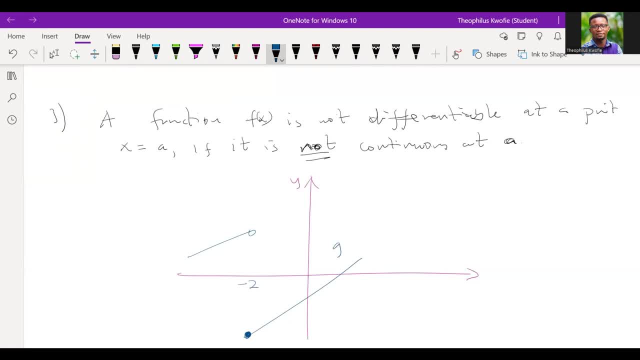 Can we say that g of x, if this is g, if such graph is g, okay, Can we say that g is continuous at minus two? Please pause the video and let's see whether we can answer this question. The question is: is g, is g continuous at x equal to minus two? 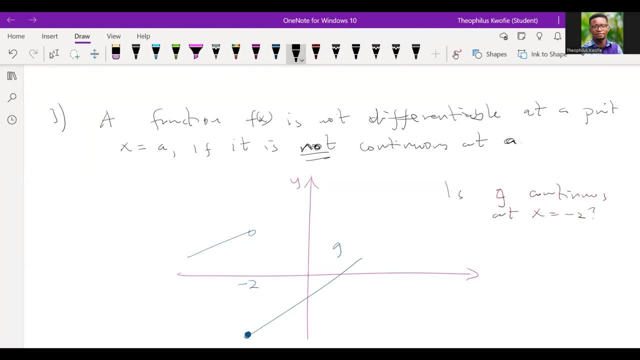 Is g continuous? The answer is what? No, It's not continuous because there's a what, There's a whole, The whole over here, the whole we see here, the whole above minus two means that the whole over here, the whole above minus two, means that there's a what. 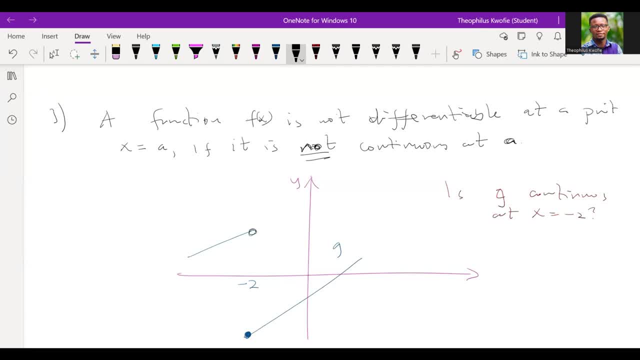 It just means there's a discontinuous at that point, so it means not continuous. So if it is not continuous, it means that if it's not continuous at negative two, it just means that it's not differentiable. So I want us to take note. 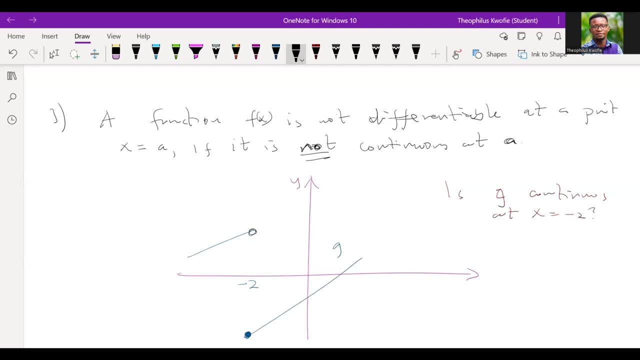 So these are very, these are some fundamental, you know, stuff that you may not want to to, to, to make. So please, let's take note, please. It's very important that we understand such things. Now, if you think you have understood this, I want us to look at this problem.